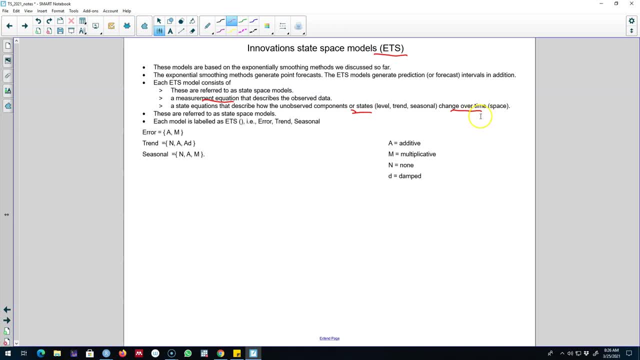 models are called state space models because they describe how a state, that is, the level, trend or seasonality, change over time or space. normally we label these models as ets, and here e stands for error, t stands for trend and s stands for seasonality. now these ets models? they can. 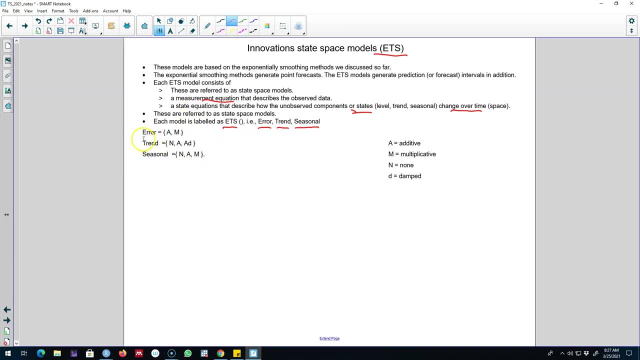 come in various combinations. for example, the error component can come either in the additive form or in the multiplicative form. the trend component can show us no trend, an additive trend or an additively damp trend. similarly, we can use seasonal component as additive multiplicative or no seasonal component. so, based on 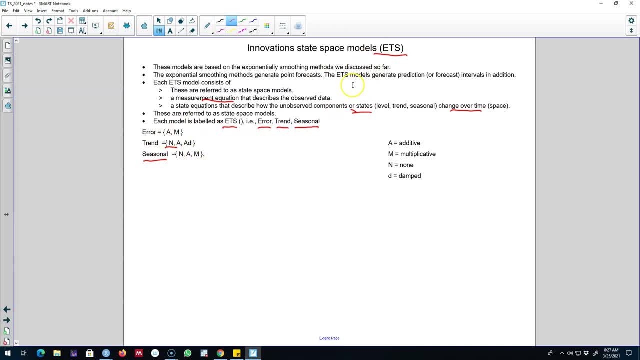 these combinations, we can build these ets models, and obviously there will be many combinations of models that we can build. so these are called innovations, state space models, and they are uh based on three components: the error component, trend component and the seasonal components. and these three components can come in uh various forms, either in the additive form, 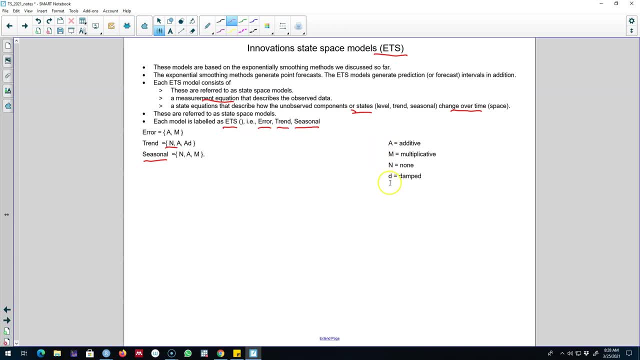 in the multiplicative form or in the non-form, and also we can introduce a damped trend here as well. so essentially, the idea here is how the unobserved components, the trend level and seasonality change over time. so we'll talk about these innovations, state space models and the idea. 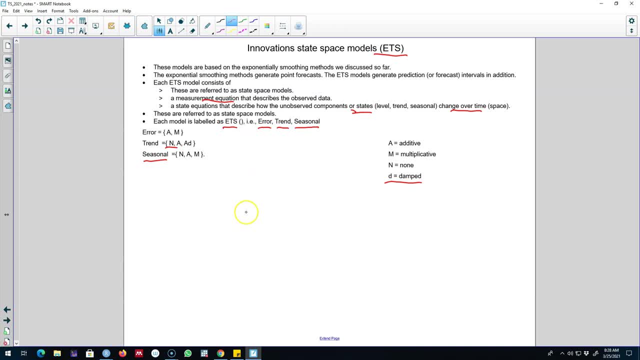 will be based on the exponential methods that we discussed so far. i'm not going to reintroduce the same equations here, but essentially, at the back of these models, we are looking at the same types of equations that we saw in the case of exponential smoothing methods. we are looking at a level 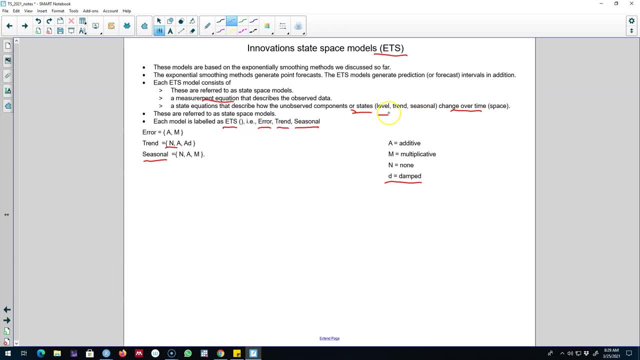 equation- a trend equation and a seasonal equation- and, essentially, there will be a smoothing parameter associated with each of these equations. for the level equation, we'll be looking at alpha. for the trend equation, we'll be looking at beta and for the seasonal component, we'll be looking 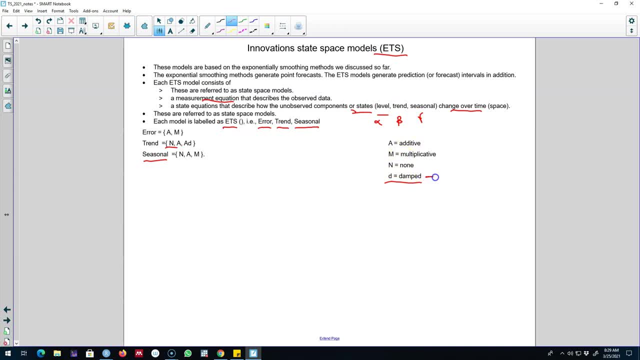 at the smoothing parameter gamma, and similarly we can introduce phi to look at the damped trend. so in the next video i'll show you how to estimate these models in r. alright, i'll see you in the next video. bye.